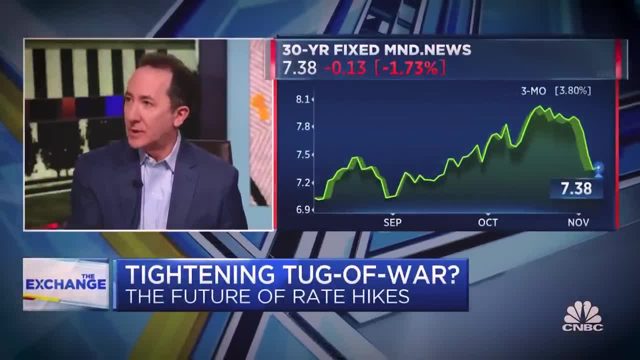 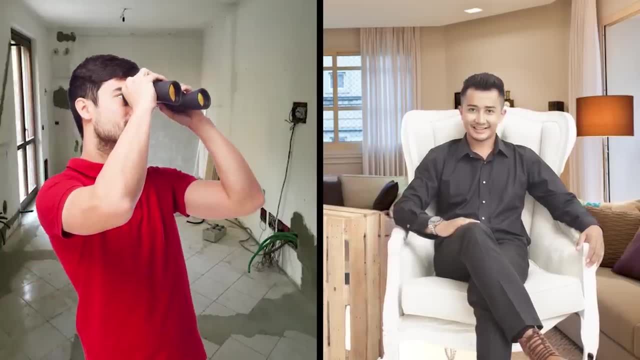 Everybody who wants to buy a home is also waiting for interest rates to fall, And everybody who is stuck renting is being forced to compete with people who already own a home but don't want to sell it because they have locked in a sweet interest rate. 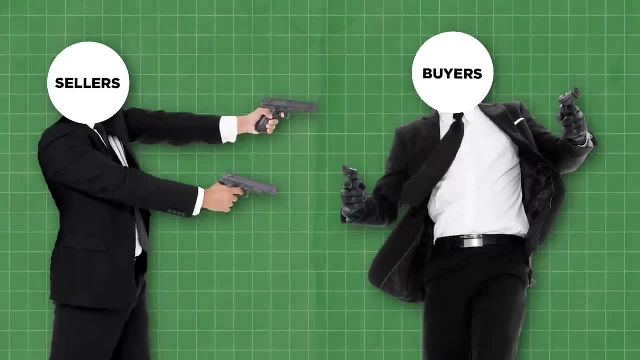 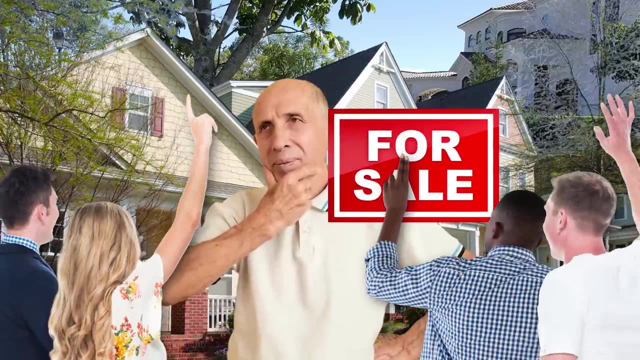 The players in the real estate market are stuck in a Mexican standoff, but the renters are stuck fighting with a banana. The only hope for people who just want to buy a home is to get it off someone who needs to sell. According to another report published by the National Association of Realtors, 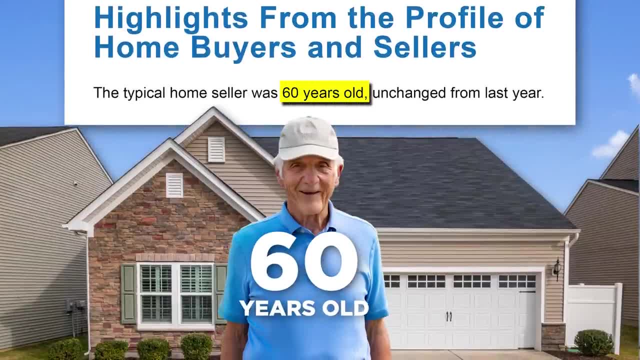 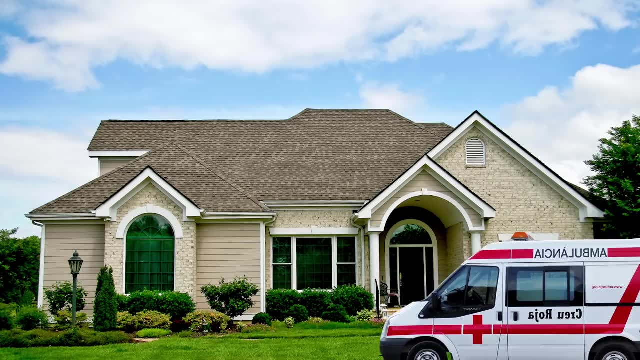 the average home seller in America was 60 years old. At that age, one of the reasons people need to sell their home is because they are dead. but if you are holding out, hope that the biggest homeowning generation in america downsizing will make it easier for people trying to buy their first home. i am here to do what i do best and crush your dreams with facts and figures. there are three reasons why older generations permanently exiting the above-ground real estate market isn't going to make it easier to buy a house. the first reason is that they can take it with them. when they are gone. the inequality between homeowners and renters is even worse in old age. according to data from lending tree, 8 out of 10 americans aged over 65 own their own home and only 19 of those still have a mortgage, the fastest growing reason why they are selling their 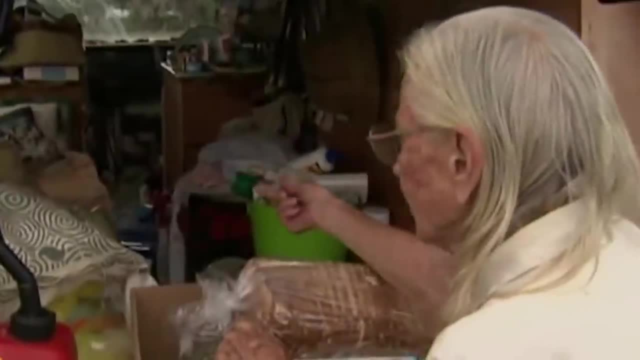 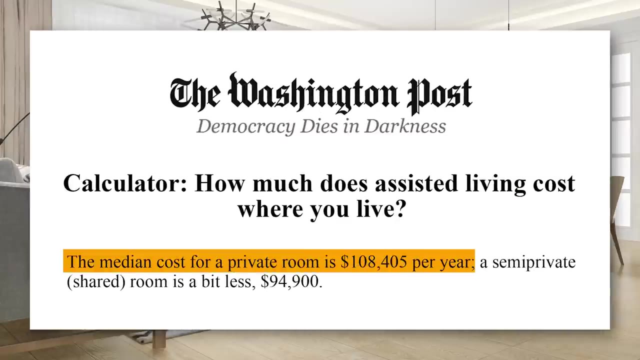 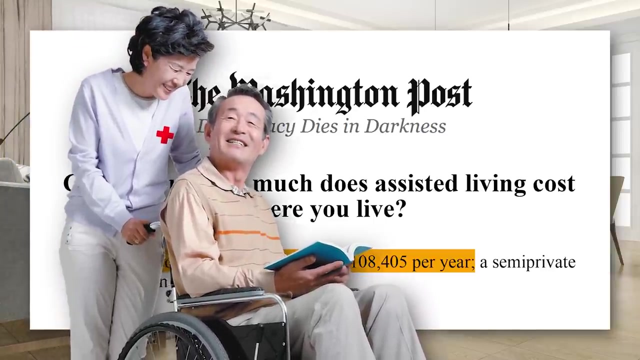 homes is not because they are dying. it's because they need money to pay for retirement living. a report by the washington post found that the annual cost of nursing homes has gone from a median of sixty five thousand dollars a year in two thousand and four to to one hundred and eight thousand dollars a year in 2020, when the article was published. 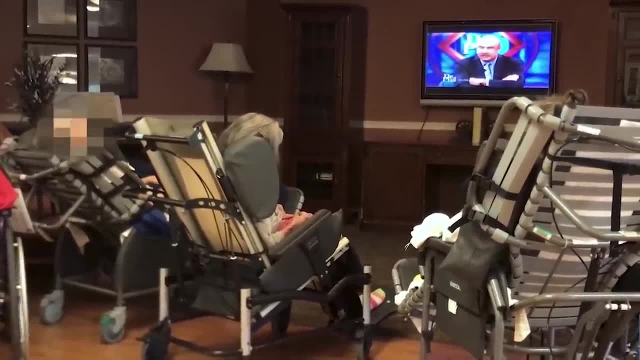 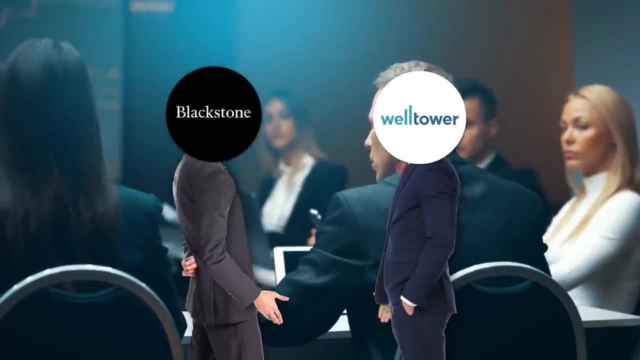 conditions in nursing homes have also been getting worse, as it's one of the fastest growing asset classes for private equity companies like blackstone and bain looking to get higher returns on real estate. in 2017, blackstone closed a 745 million dollar deal with the real estate. 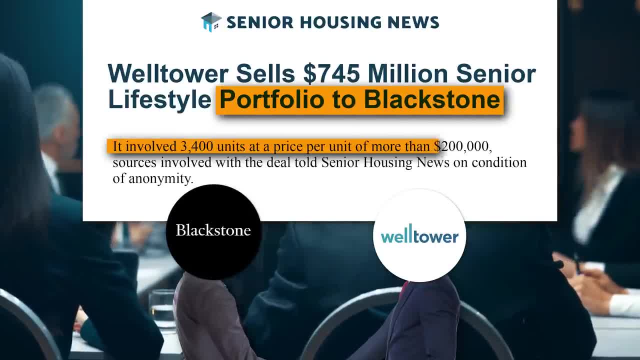 investment trust well tower to buy its portfolio of 3 400 aged care units. blackstone's holdings are growing, but they are dwarfed by other private equity firms that have raised their homes for the first time in over a decade. blackstone's holdings are growing, but they 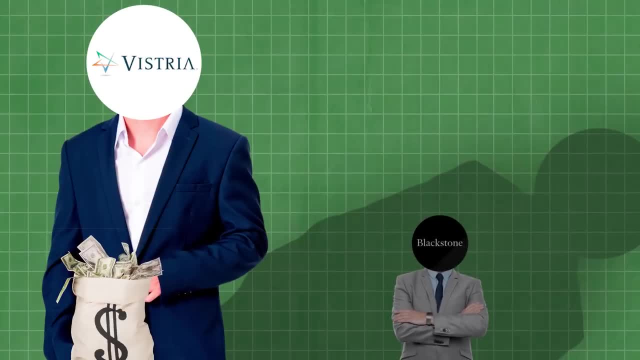 are dwarfed by other private equity firms that have raised their homes for the first time in over a decade. blackstone's holdings are growing, but they are dwarfed by other private equity firms billions directly into aged living because they know how much value it offers investors. 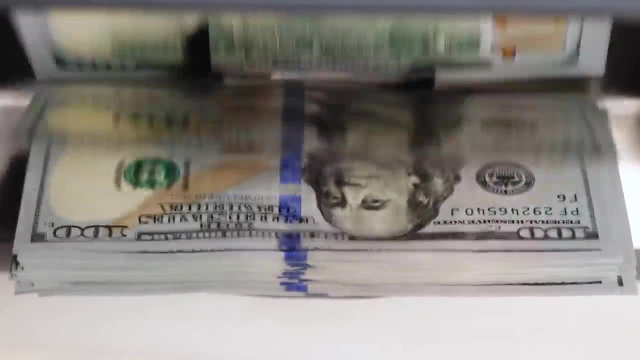 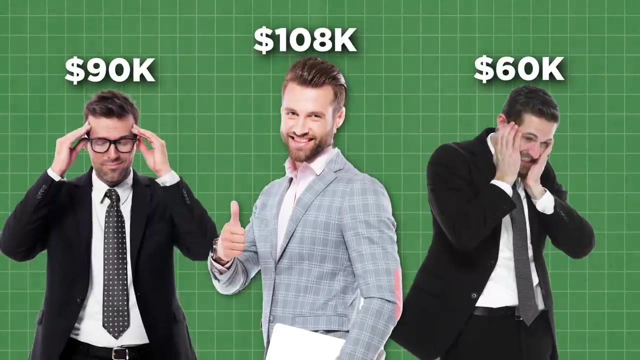 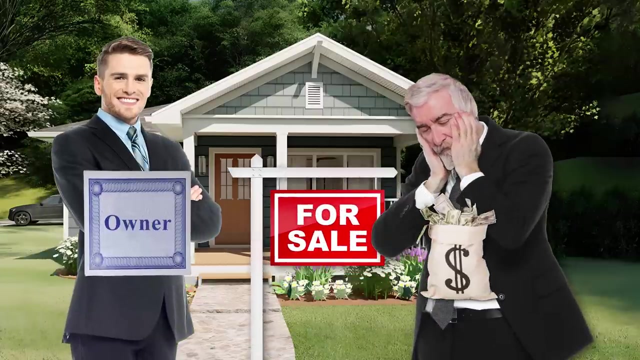 by cutting costs and raising prices, these companies have generated exceptional yields off real estate developments that cater to a growing market of elderly americans. most americans don't make a hundred and eight thousand dollars a year, and even fewer can afford that much in retirement, so people are selling their homes to pay their fees to these facilities. 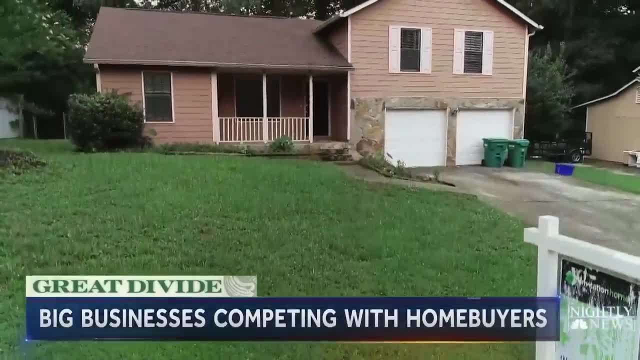 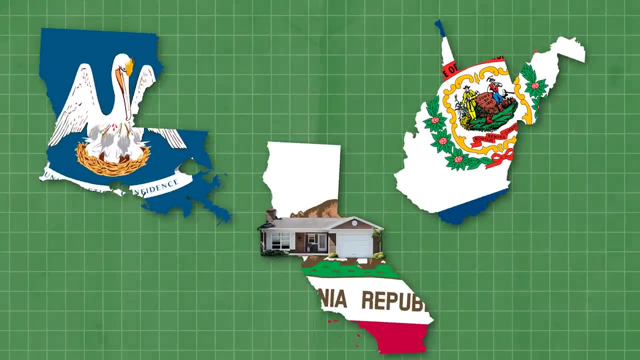 private equity's role in buying up single-family homes away from regular families is overstated. but they have realized that they don't even need to own the homes to benefit from their value. states where home prices were highest had the most expensive aged care facilities because elderly residents in those states have more money to pay for it. 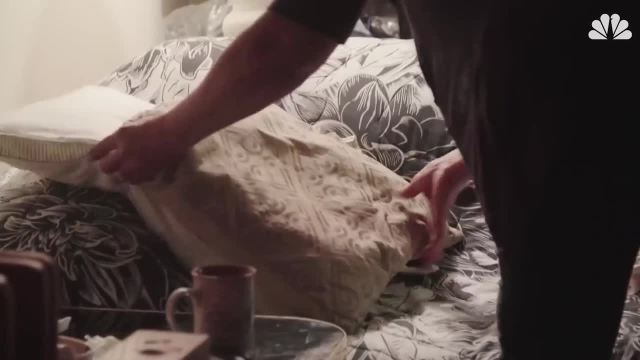 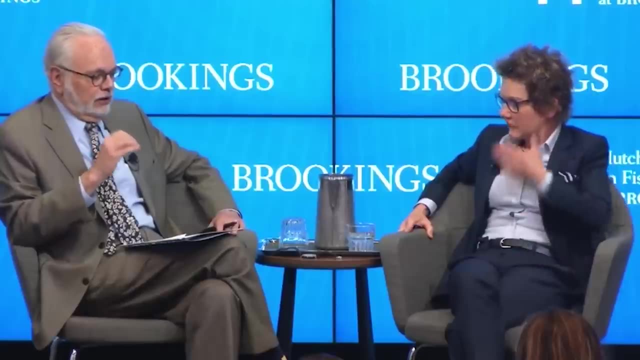 after selling their homes. people that can't afford to pay these fees are relying on limited social security and their own family and friends to support them when they can no longer physically work. according to federal data and a 2020 brooking study, slightly more than 10 of american adults. 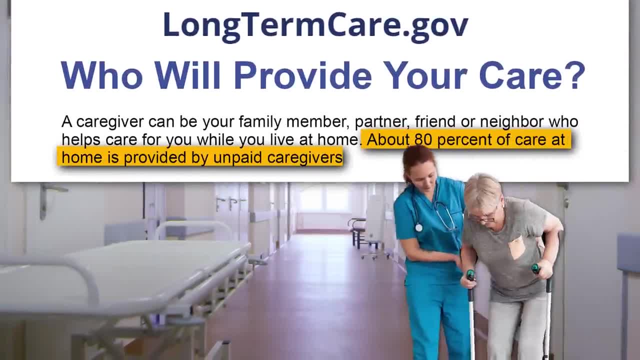 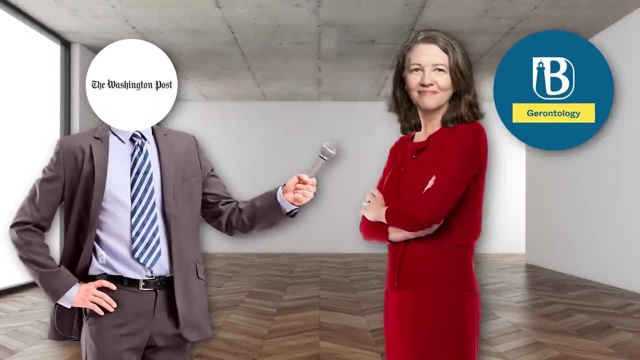 provide some type of care to another adult. usually it is an adult children caring for their parents. in an interview with the washington post, jan mutchler, a director of the gerontology institute at the university of massachusetts, said that when an adult child takes on those roles a lot of times 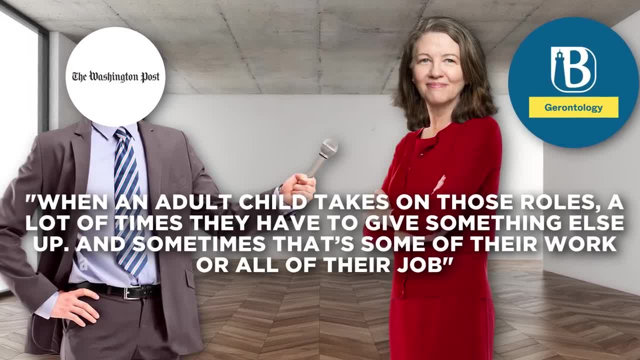 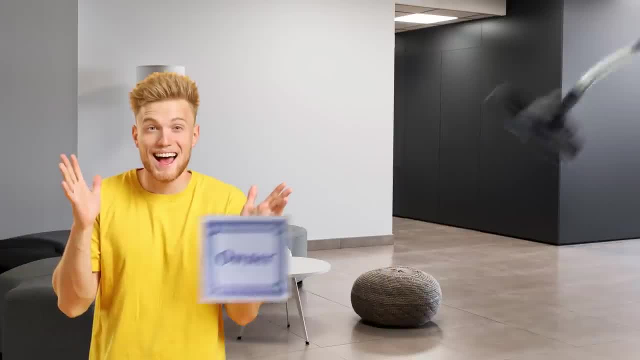 they have to give something else up, and sometimes that's some of their work or all of their job. so if you are waiting for that inheritance to finally buy your first home, it's just as likely that this wealth will be sucked up by private equity companies before it gets to you, and that's 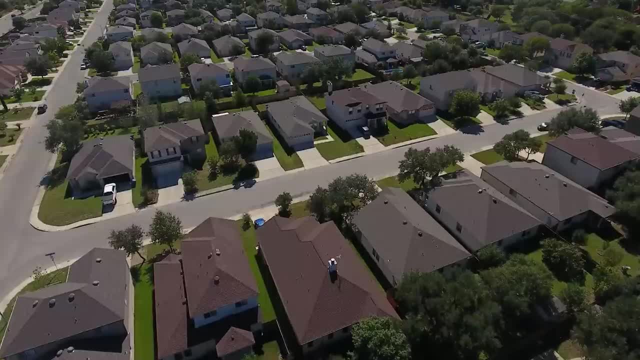 just the first reason. so it's time to learn how money works, to find out why you probably won't benefit as much as you do if you're looking for a home that's worth more than a thousand dollars, much as you are hoping, from the boomers passing down their homes. this week's lesson was sponsored. 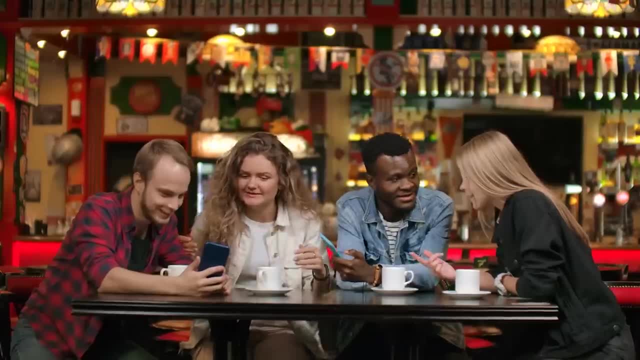 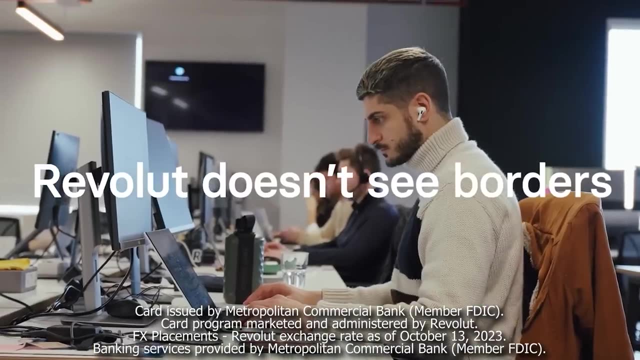 by revolut. revolut is a global financial super app used by over 30 million users that gives you the tools to easily save, spend and invest your money. my team and i work from all over the world and we found revolut to be useful for our personal and business needs. 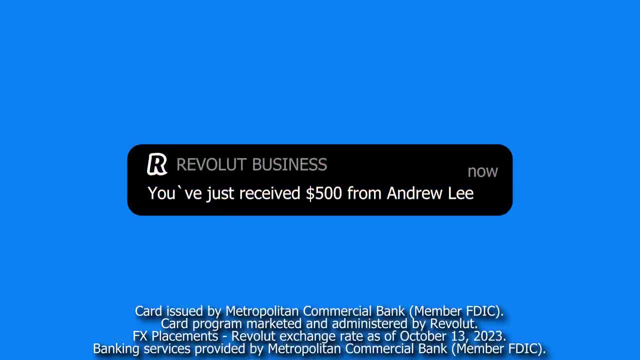 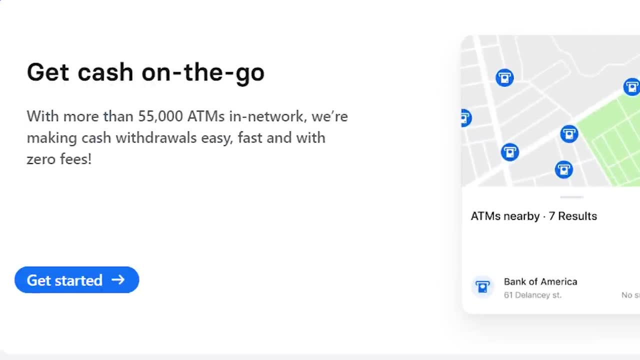 why they offer multi-currency accounts with low fx fees, making it easy to send money worldwide with little to no fees. plus, when you travel, you can withdraw cash with no fees from over 55 000 atms globally. revolut makes it easy for us to send money peer-to-peer in over 40. countries. choose the revolut plan that fits your needs standard, which costs zero dollars per month, premium or metal. i've been using the metal plan for over a year now and i love it. start using revolut today by using my link in the description. the average age of a first home buyer in america. 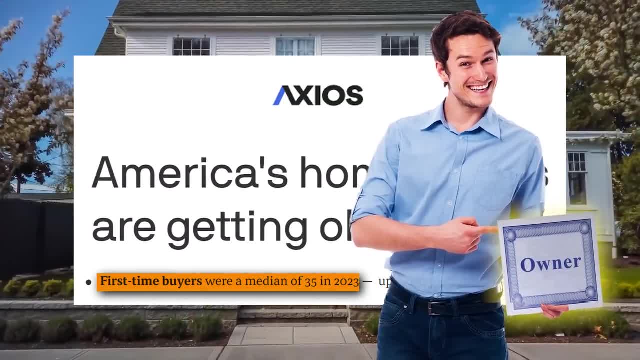 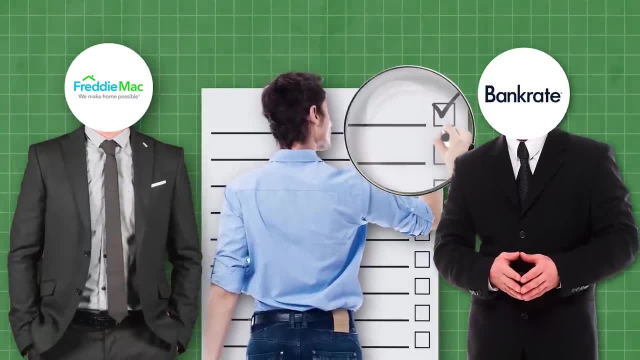 is now 35 years old, up from 33 years old in 2021 and just 30 years old in 2010.. the survey of young home buyers conducted by freddie mac and bank ray asked why young people were waiting until later in life to buy a home. i probably don't need to tell you that the number 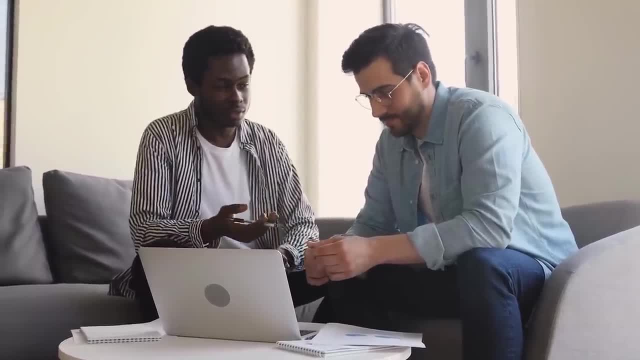 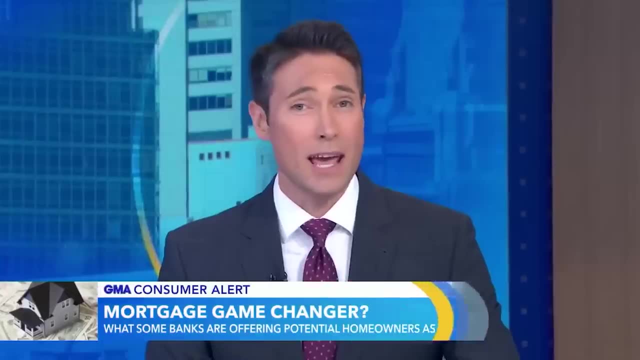 one response was that people wanted to buy their first home sooner, but they couldn't afford it until they had paid off their student loans, progressed in their career and had dedicated years of saving a down payment. new financial products that offer home lending with lower down payment requirements have been ruled out by banks, non-bank lenders and the government. as an answer to this problem. the average down payment of seven percent means that some first time home buyers are contributing significantly less to their first purchase by using products like the federal housing administration loan insurance, which allows first-time buyers to put down as little as three percent of the purchase price plus closing costs companies 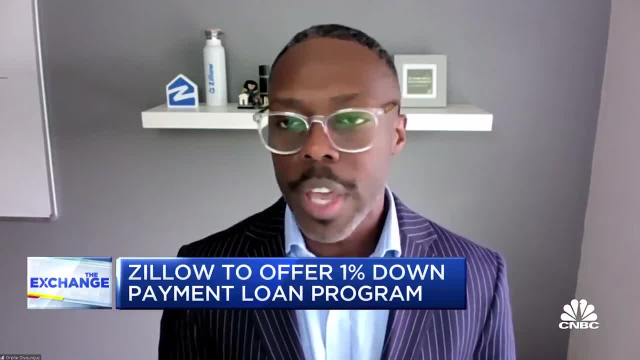 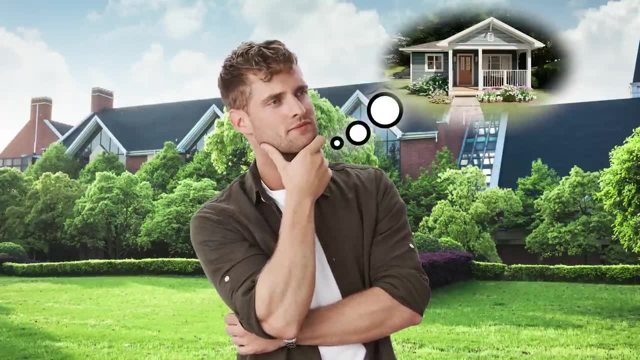 like zillow, are taking this a step further with plans to roll out one percent down payment financing to eligible home buyers nationwide. if you are someone who wants to buy their first home, these offers may look like they are there to help you out, but they are actually just making. 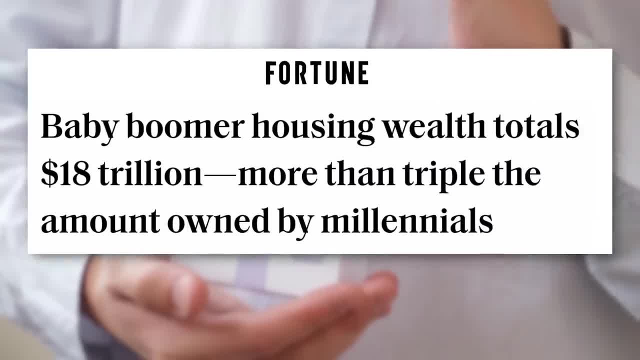 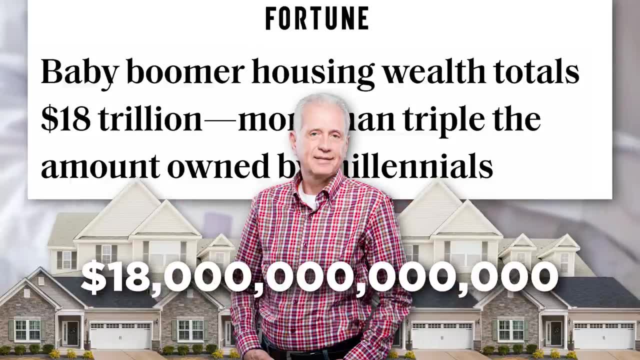 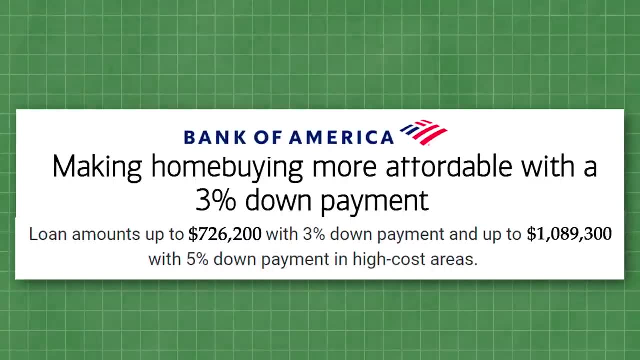 the problem even worse. the only people these lending products are really helping out are the people who already own multiple properties, which, according to redfin, are mostly baby boomers who own 18 trillion dollars worth of real estate. according to the disclosures of these loan products, most offers have a limit on the total loan size that can be taken out. these 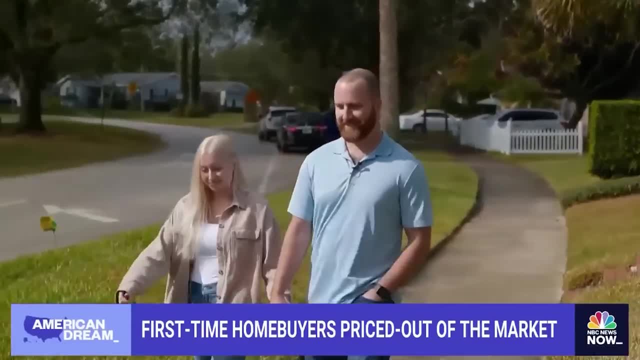 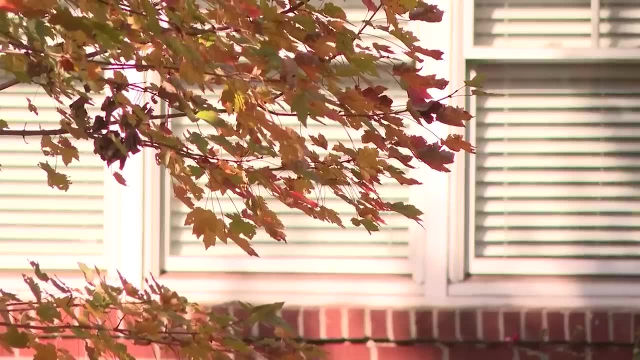 products are meant for first-time home buyers who want to buy a basic home, so that's fair enough, but all that it really does is pump up the price of affordable homes until they become unaffordable again in an even worse way. what these loan products do is move the financial bottleneck. 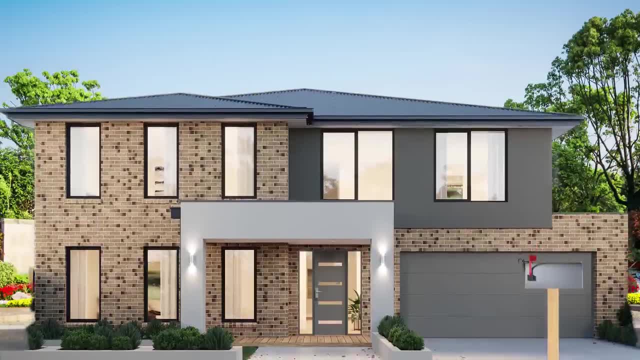 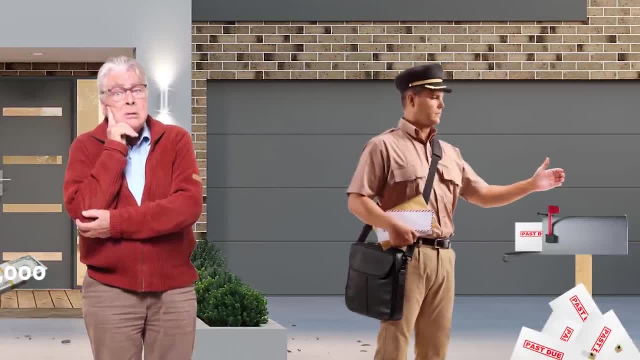 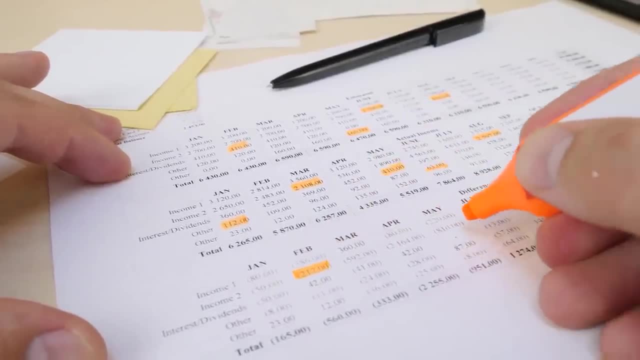 ten thousand dollars down doesn't mean they'll be able to afford the repayments. a down payment is a one-time expense, but repayments on a house that is more expensive than it should be because of a loan product like this have to be paid every month for the next 30 years. the only real winners. 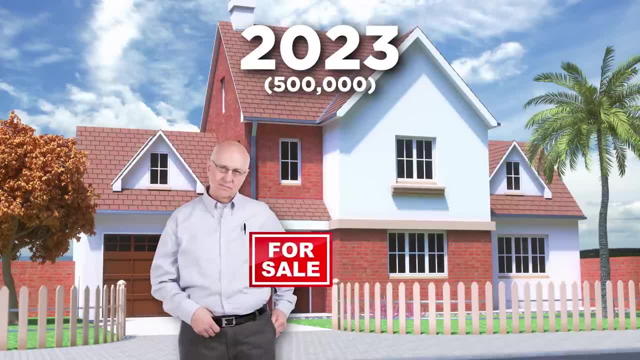 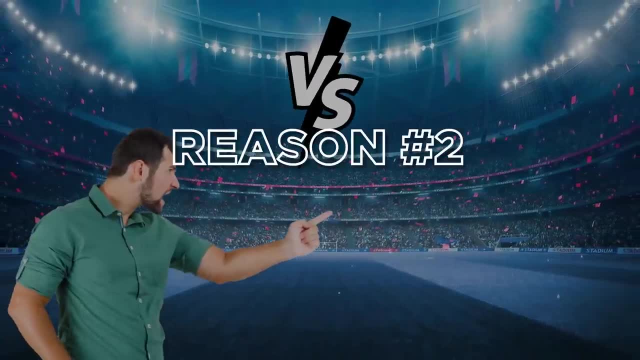 are the people that purchased these homes when they were a quarter of their current value and can now sell them to buyers with risky financing. and that's the second reason why boomers retire from life isn't going to make it easier for you to find a home. it was never a matter of age. 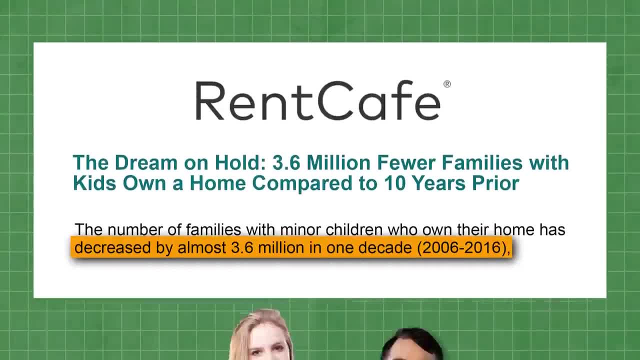 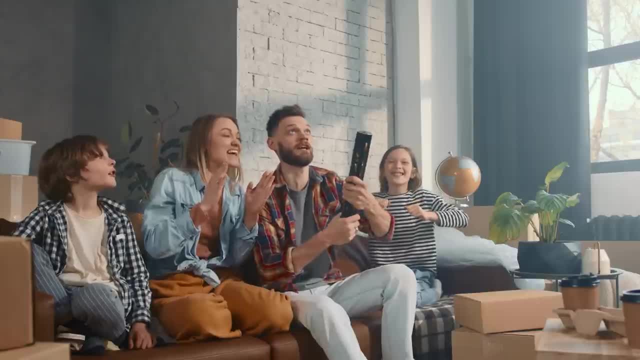 according to the us census bureau estimates from 2016, the number of families with children who own their own home decreased by 3.6 million. in the 10 years prior to the survey. families with children were preferring to rent either because of the flexibility. 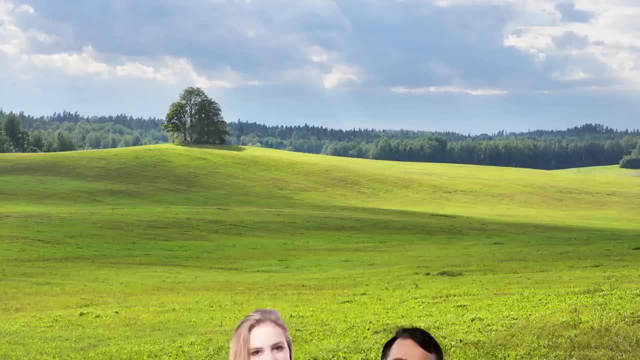 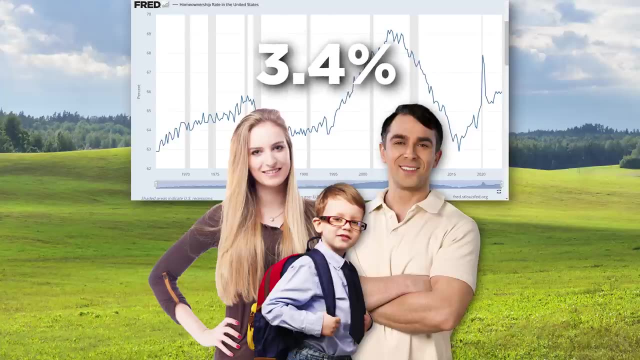 offered or because they could not afford to buy their own home. families that own their own home also have fewer children on average, and the overall national home ownership rate has decreased by three point four percent. however, the small number of families that own multiple pieces of real estate. 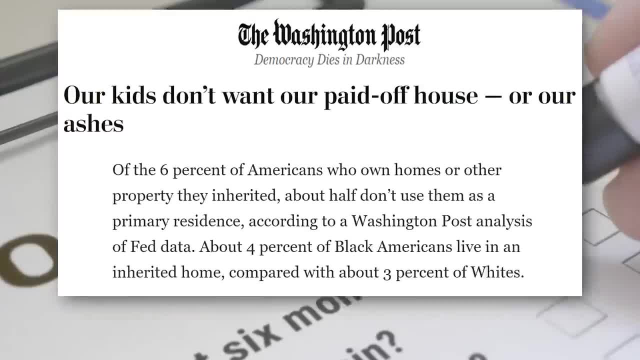 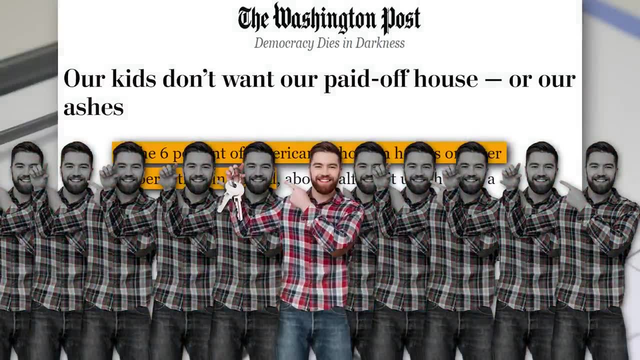 as rental properties or holiday homes is growing. according to the 2022 federal reserve survey of consumer finances, only six percent of americans own property that they inherited and only three percent live in a property that was passed down to them. the other homes are being kept by a small 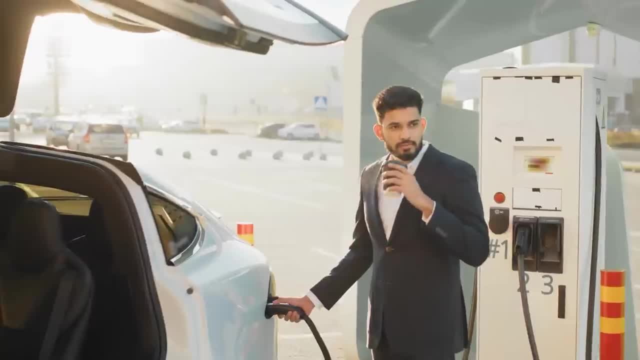 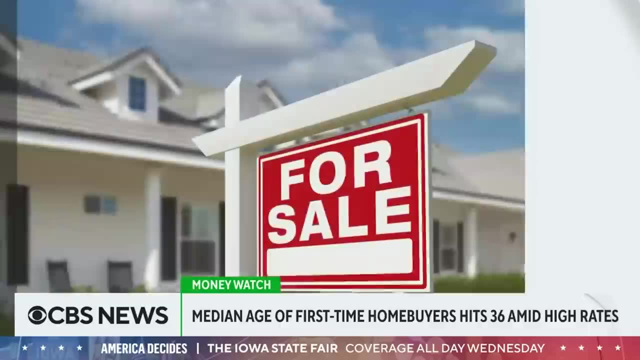 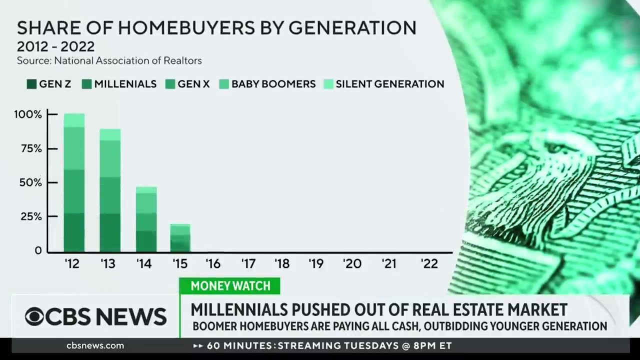 handful of children from wealthy families as investment properties, often in addition to the homes that they already own themselves. so if you think, you just need to wait out the boomers to afford a home, unfortunately the statistics say that their estates are only going to become more concentrated in the hands of fewer people. their age doesn't matter, but their wealth does. an article. 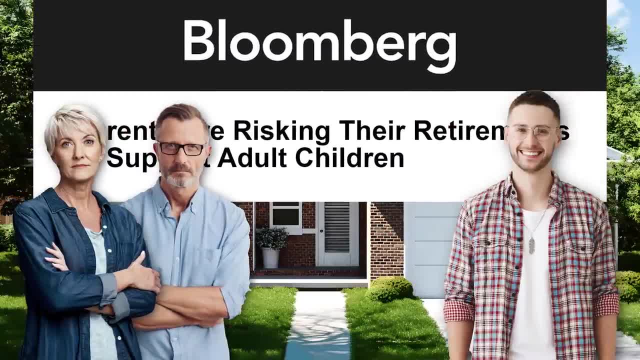 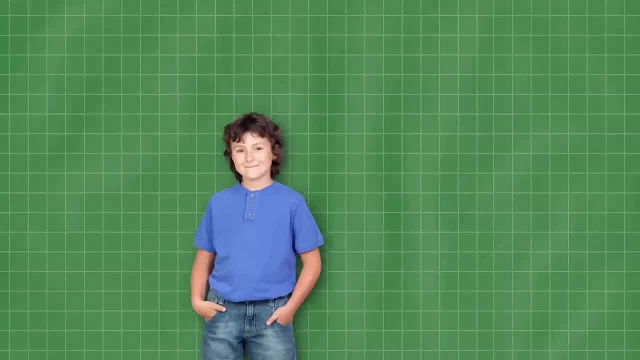 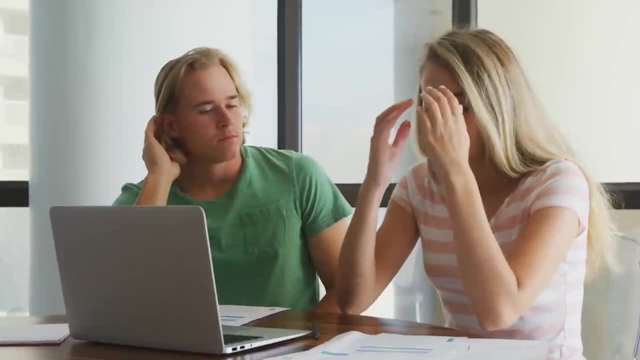 by bloomberg surveyed people with adult children and found that a majority of respondents reported draining their own retirement savings to support their children who are struggling to afford a home to live in. some families are going to leave multiple homes to a few children. some families are going to make big sacrifices to help their children. some families don't have enough to help. 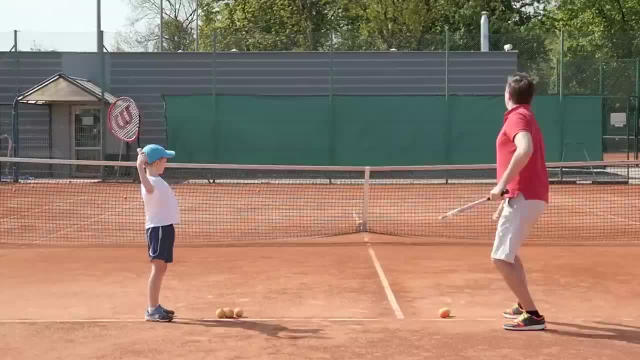 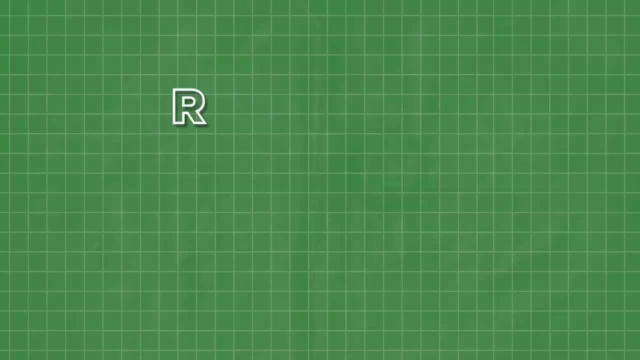 and some families are going to need support from their children. if you are not a part of the first two groups, then you are going to be even further behind when assets are passed down from older generations, and that's the third reason why you shouldn't hold out hope for a flood of new houses. 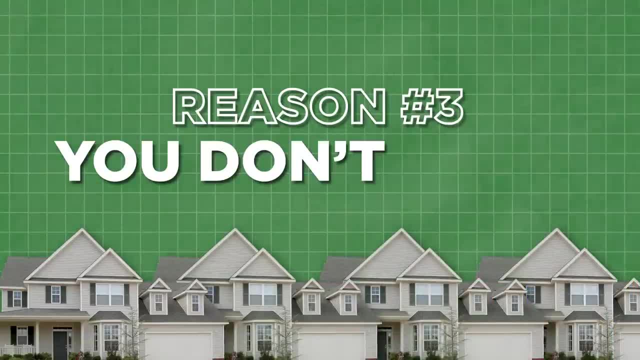 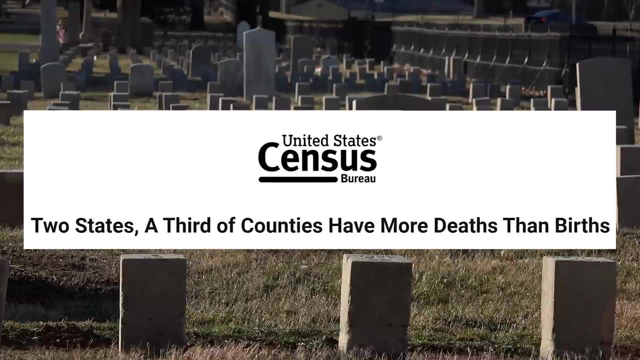 hitting the market. when all the boomers die, they aren't leaving houses for you. a 2017 census report found that a third of counties in america were experiencing more deaths than births. states like florida have a lot of old, wealthy retirees that have displaced normal families in 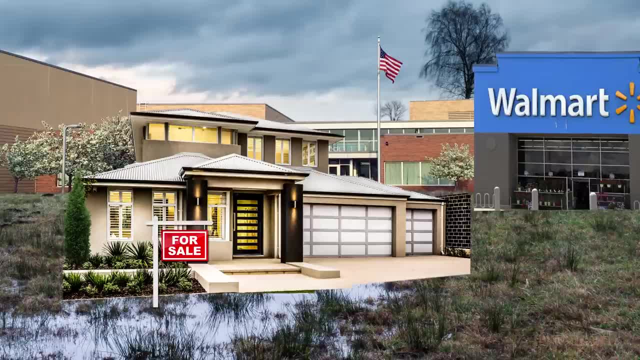 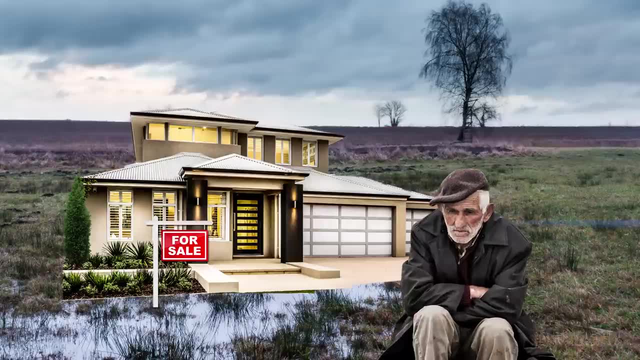 communities. the homes that are being left in these areas don't have the amenities that first home buyers want, like access to job opportunities or good school districts, because retirees pick places to live to avoid these things if the people who inherit these properties don't want to live in a 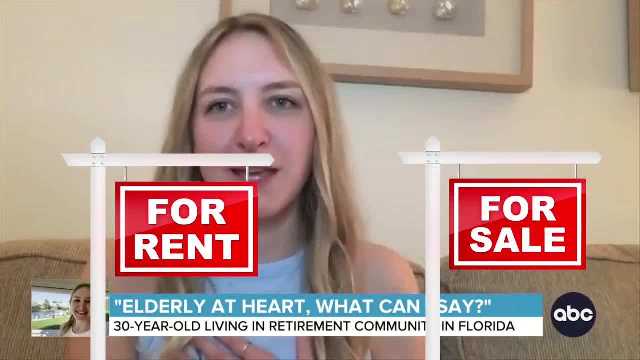 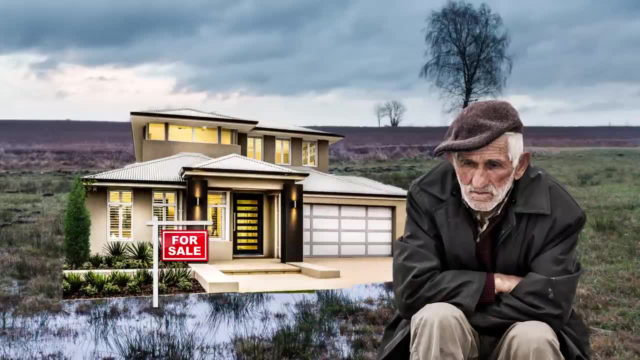 community full of retirees. they can either sell the property or rent it out. if they sell the property, it will add supply to the housing market, but it won't be in an area where a first home buyer wants to purchase. according to the state of housing published by harvard university institutional,